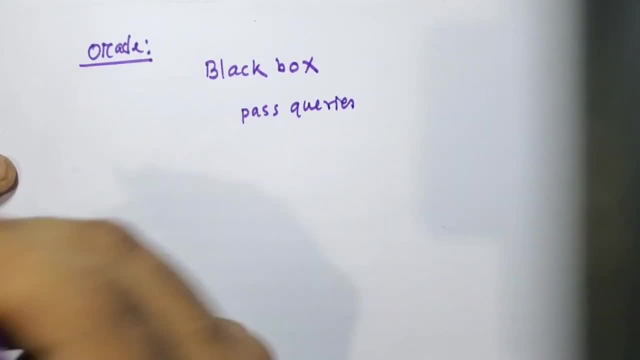 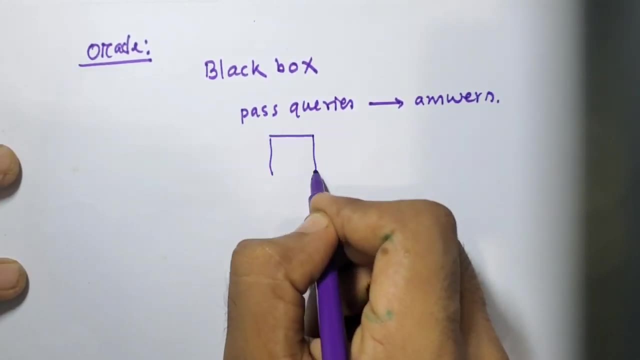 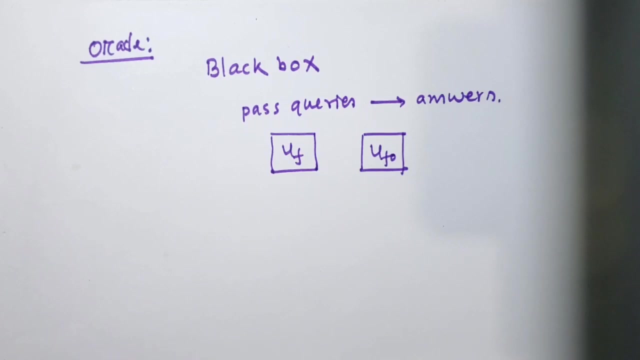 queries and watch return answers and get answers. These are mainly oracles and black balls. These are physical devices. In Grover's algorithm. we have two oracles mainly used, which we will discuss later on. So first let's see the circuit of Grover's algorithm. 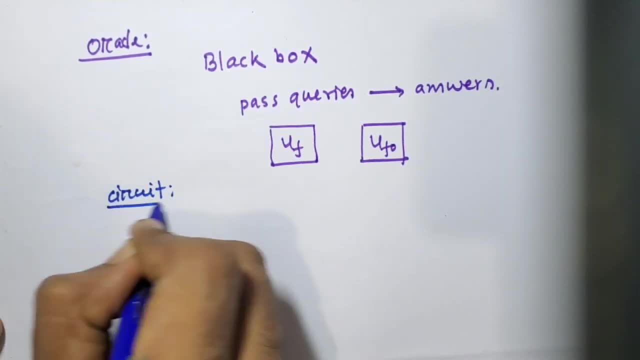 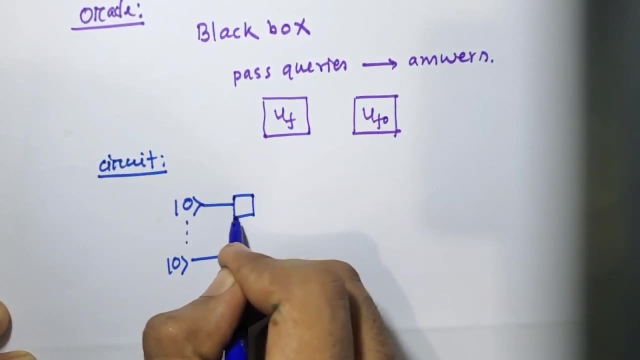 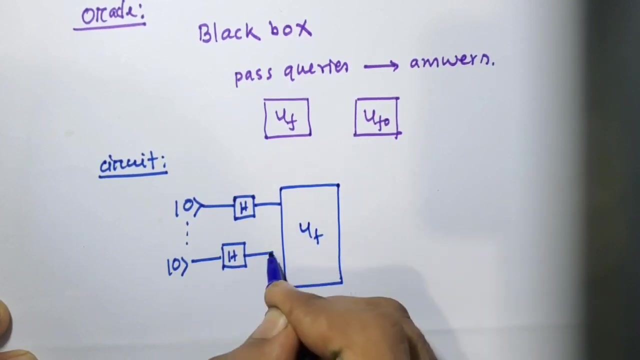 The circuit goes like this. Here are our qubits. First we pass them into a Hadamard gate for uniform superposition. Then we pass them into our first oracle. How and what these oracles does, we will discuss later. Then again a set of Hadamard gates and now the 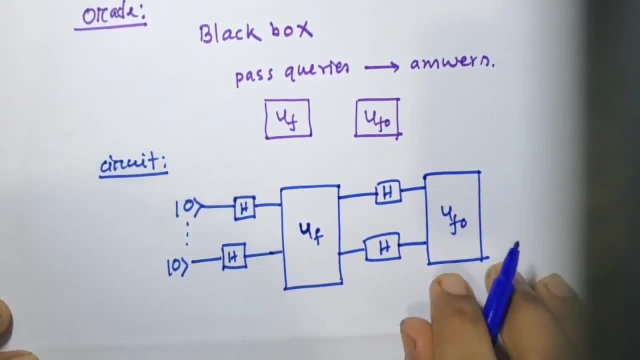 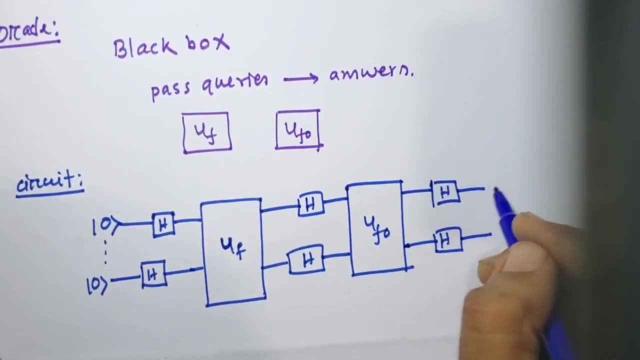 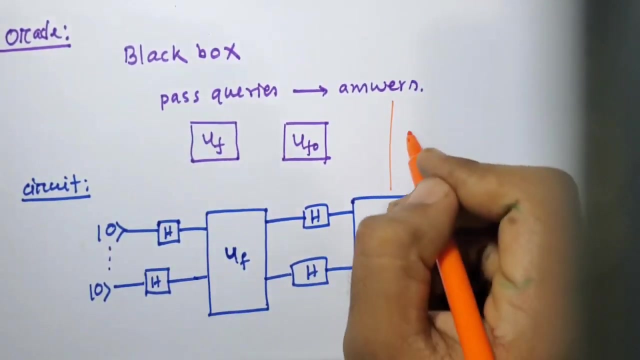 oracle, Second oracle, After that, we just measure these things and get our output, the result. This is the main circuit. So what was the claim in Grover's algorithm? The claim was to find w with high probability. If there are n elements, we will find them within the order of square root of n. 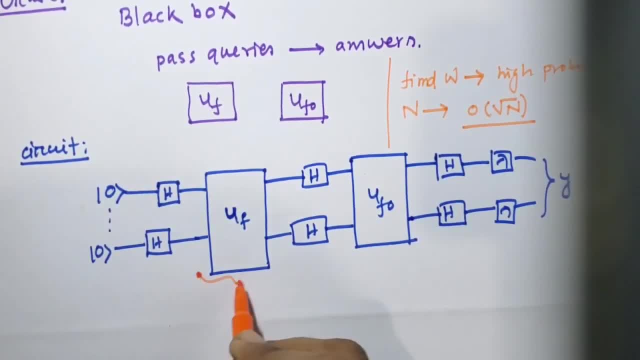 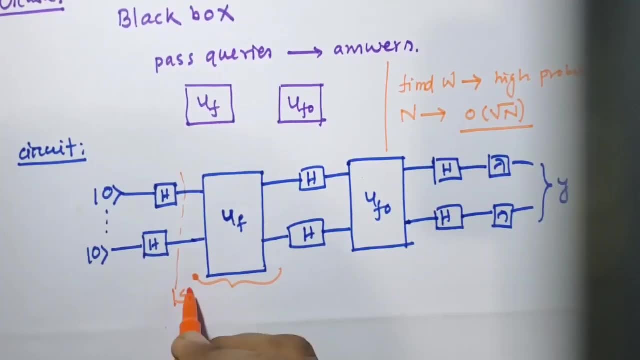 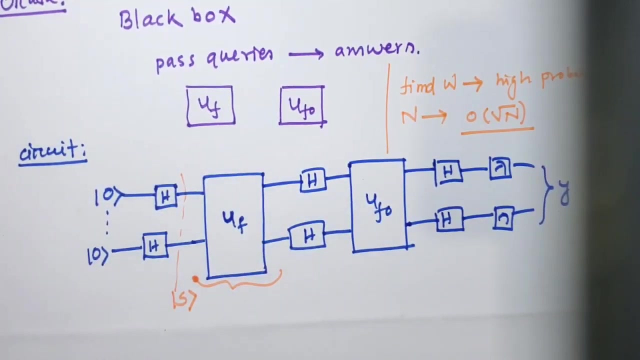 Here. this is the first oracle where we pass all the values Before that we get this state, the s state, which is the superposition of all the states, And when it goes into the oracle, this is a mainly phase inversion oracle. 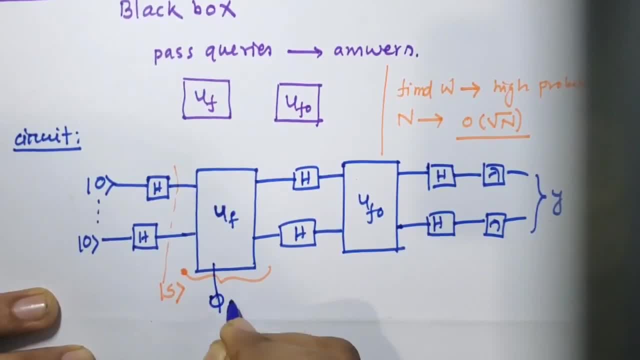 What this does is inverse the phase, Phase inversion, So it changes only the phase of w. If the input is w, it goes to minus w, And if it is anything other than w, it stays the same. x not equals w. 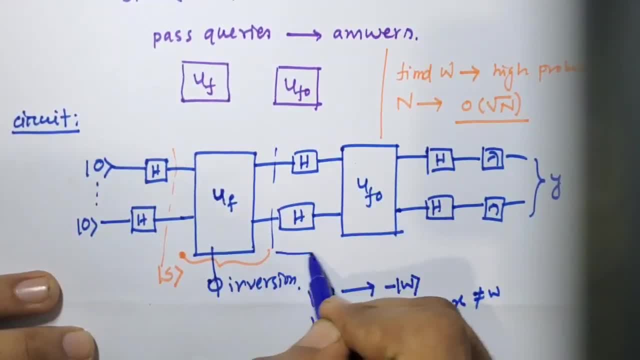 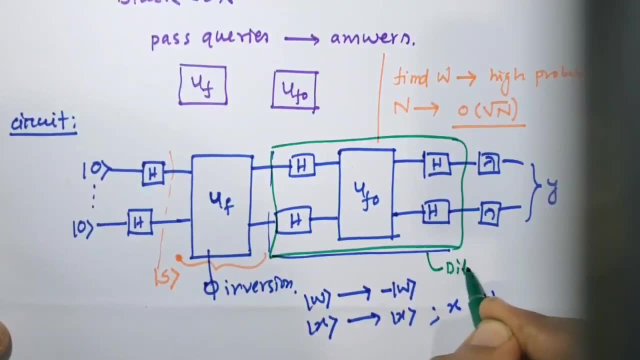 Now, after passing from this, here comes this state. This is called the diffuser. Let me mark it green. This is a diffuser. The total system is v, And mainly if there are square root of n evaluations, that happens here. 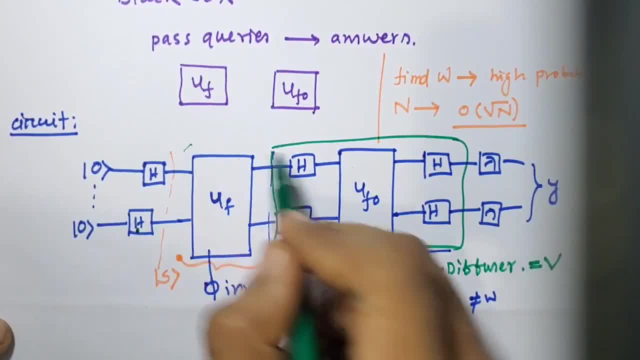 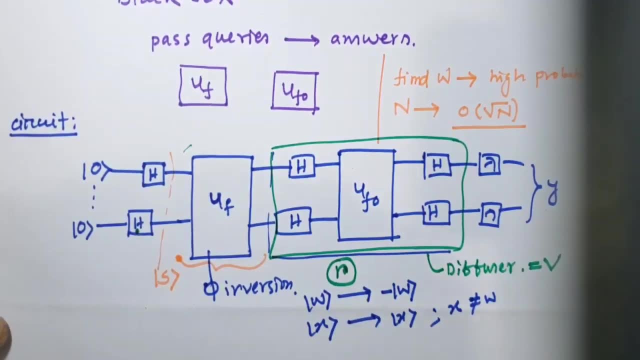 We do this, this Heidelberg gate and this oracle and this whole system. r times r is the number of evaluations we need to do. That's square root n. These are both are the same. Now let's dive into the protocol and all the states of the algorithm. 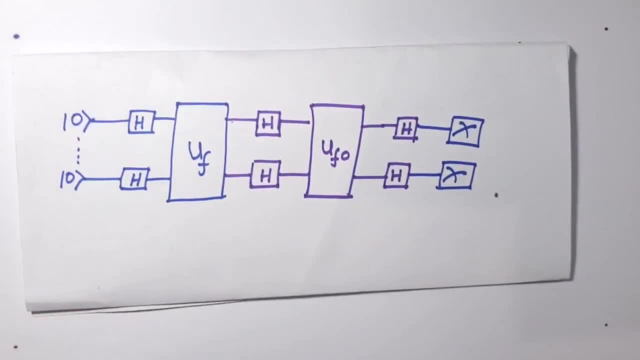 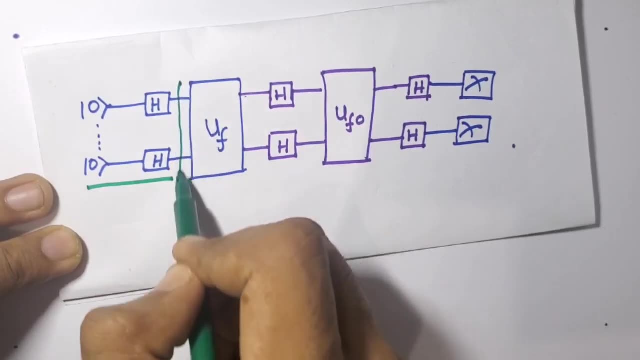 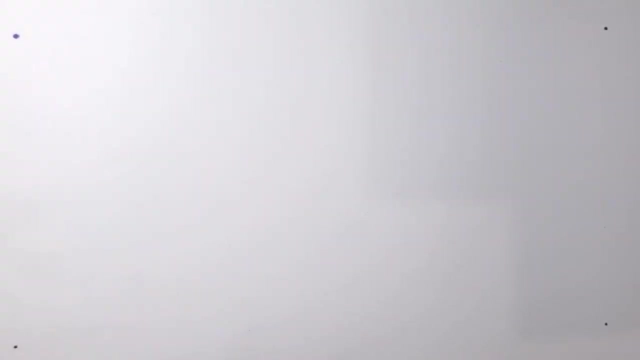 In the first step. what we will do is: this is my circuit of the Grover's algorithm. Now here- this is my first step. I apply Heidelberg gate on all the states and I name this state the s. So what actually happens is the Heidelberg gate creates an uniform superposition on all the states. 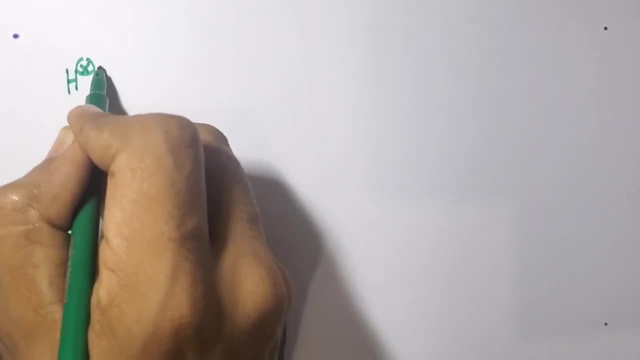 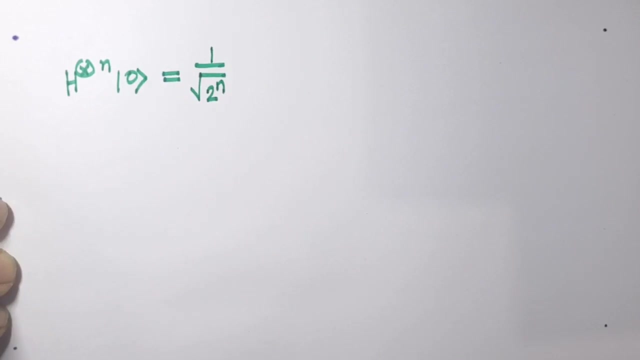 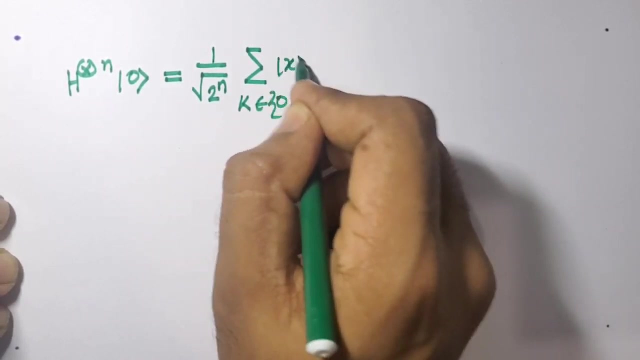 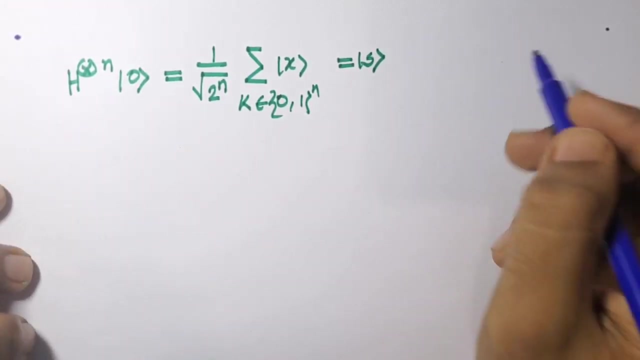 First of all. so if I apply this, this means all the states to the power n have equal amplitude and it belongs to x and this- I name this- the state s. So here, if I draw this for better understanding, in this side I have the amplitude. 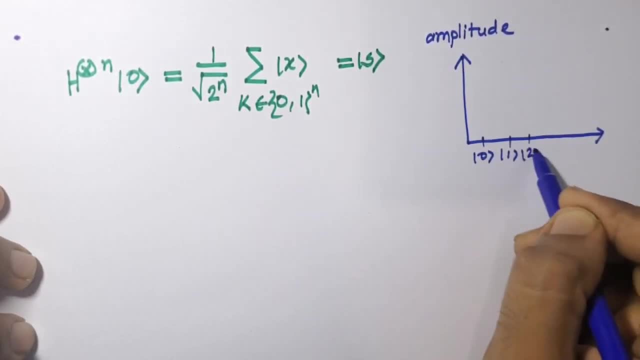 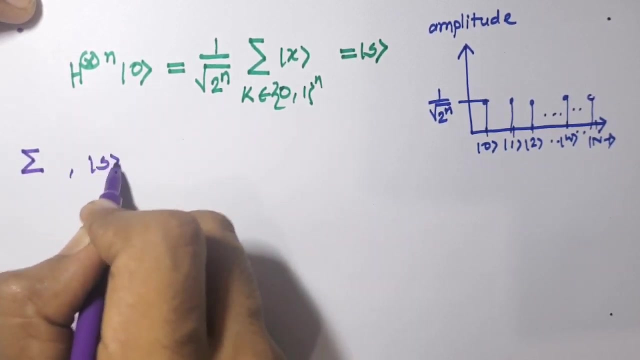 and here are all the states: 0,, 1,, 2, w dot n minus 1,. all the states and all, have equal probability, Which is 1 over root 2 to the power n. Now let sigma be the space spanned by s and w. 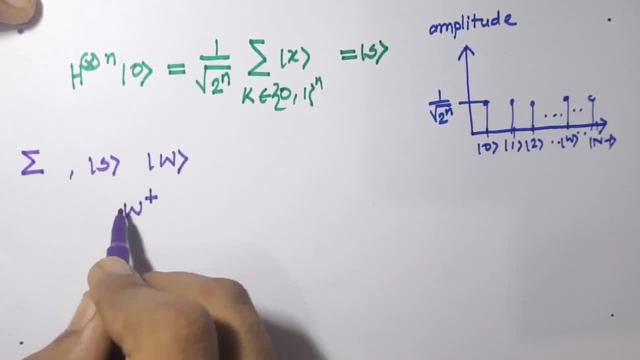 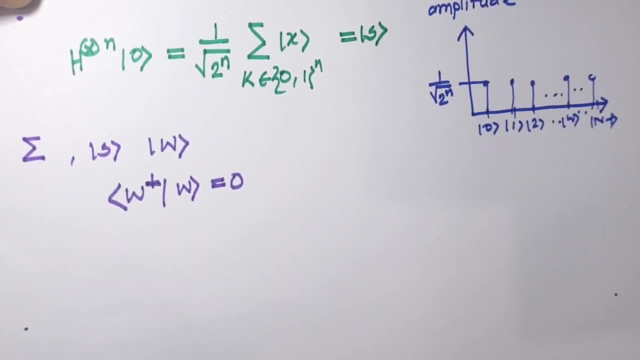 And we define w perpendicular, such that its orthogonal is perpendicular to w, and inner product of these two is 0. So w is like the vector, It's all other values except 1, which is w. So x not equals w. 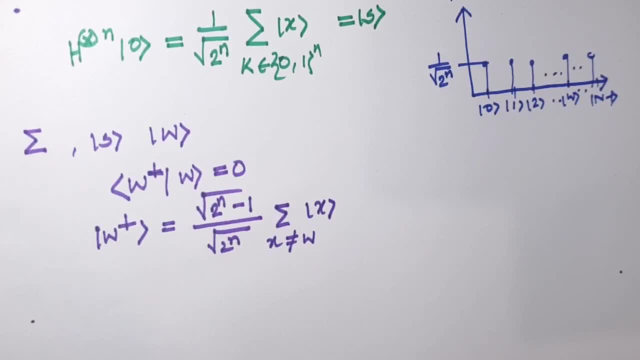 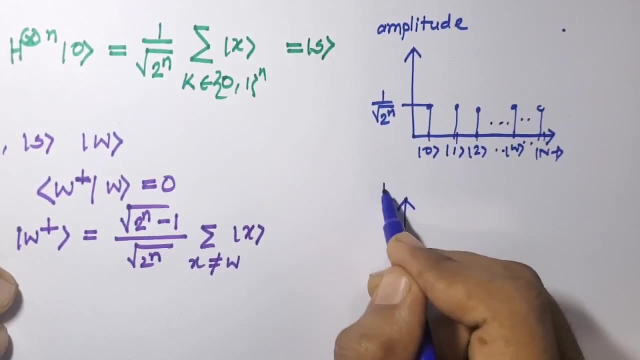 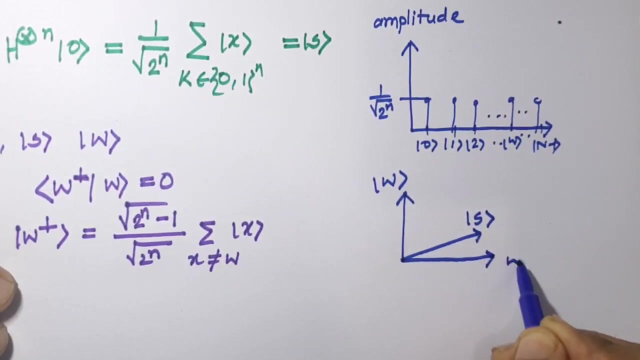 This is my w perpendicular. So if I try to draw this, what I will get here is my w and this is s. And since w perpendicular is orthogonal to w, it will go something like this: Now, if I write s: 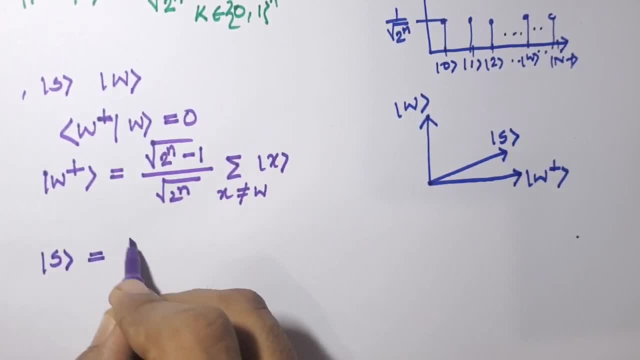 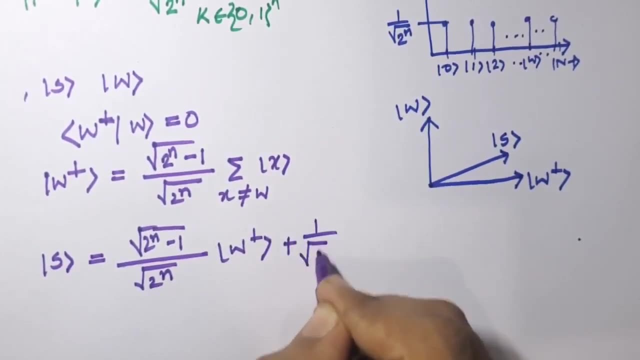 as a projection. I can write this as: root of n minus 1 w. perpendicular plus 1 over root n w. This is my s, And I can further write it this as cosine of theta by 2.. That's why I'm defining this plus sine of theta by 2.. 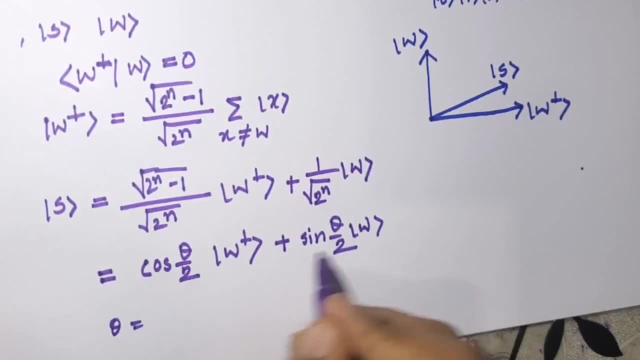 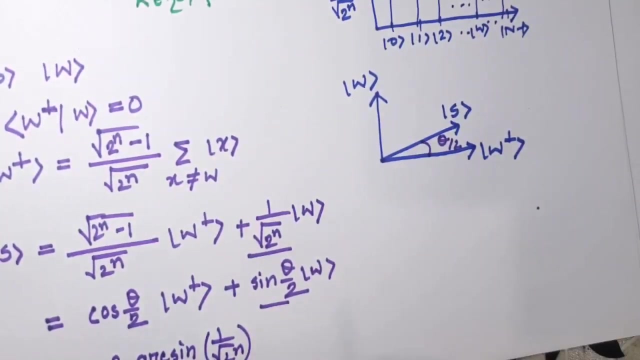 Where theta is comes from this and this. Here and here I get 2 r sine 1 over square root of 2 to the power n And theta by 2, this is theta by 2.. So s is projection onto this one and this one. 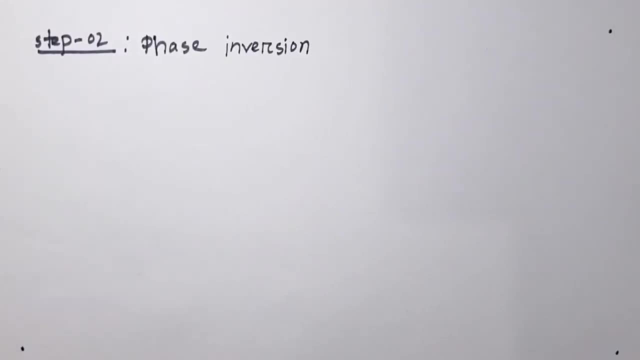 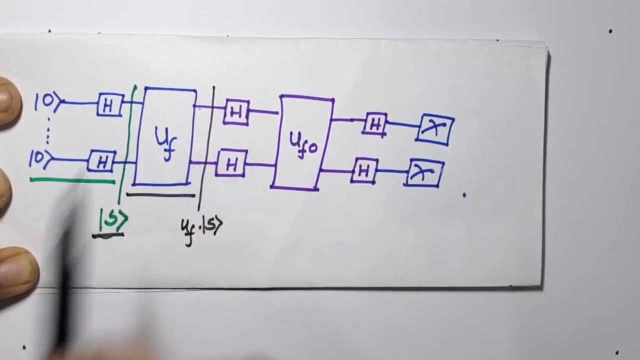 Now we will see the second state, which is phase inversion. This happens here, In this state, after the uniform superposition state, we apply this oracle, this black box, And this inverse, our phase. So how does it work? 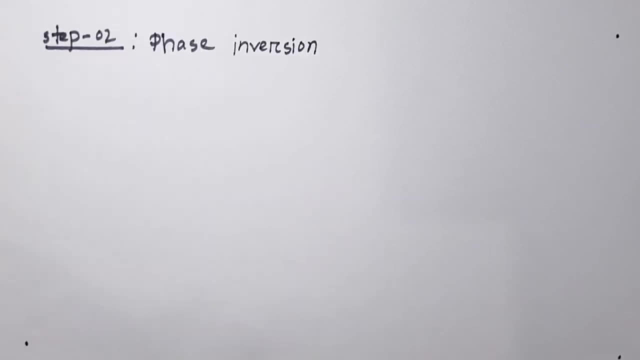 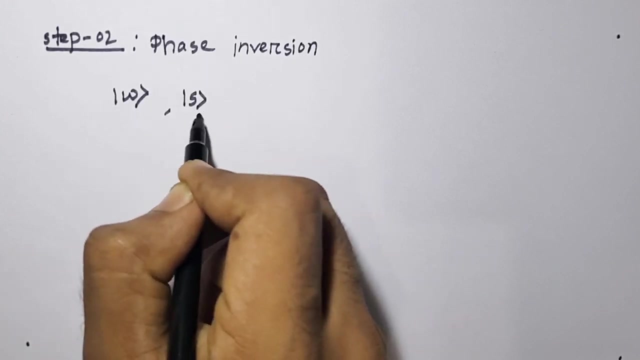 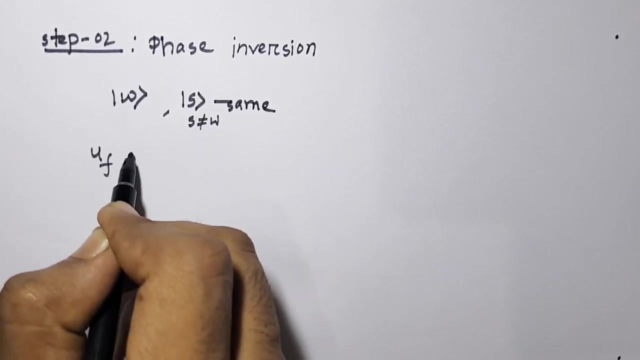 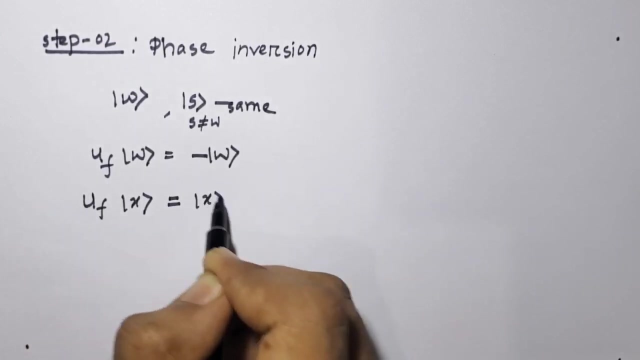 Actually what this does is it changes the phase of w only and gives the other states of s where s not equal to w same. So uf on w state is equals to minus w, But uf on x- any other state- is equals to x. 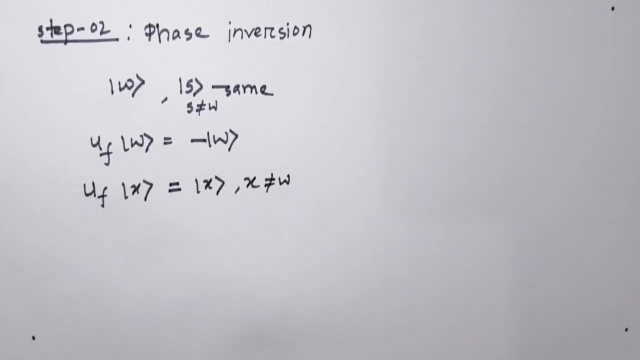 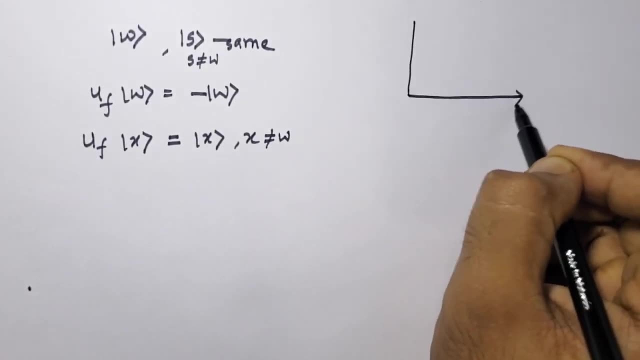 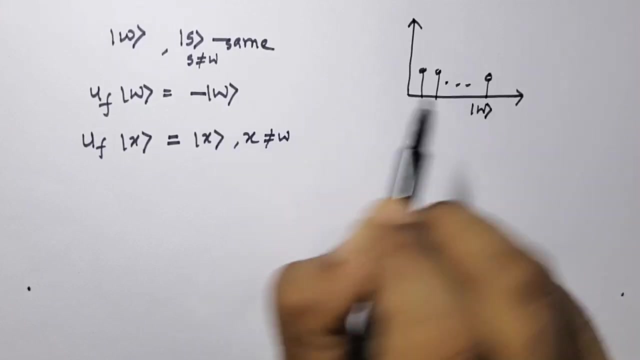 Where x not equals w And to draw the picture, all the other states are like this: Here is amplitude and these are my states. This is my w previously, But now it is shifted in this way: This is my new w and this is normal. 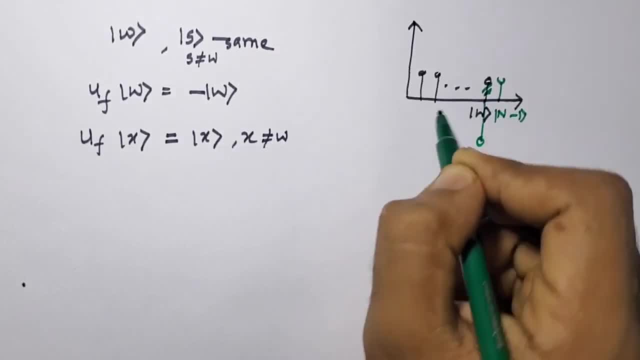 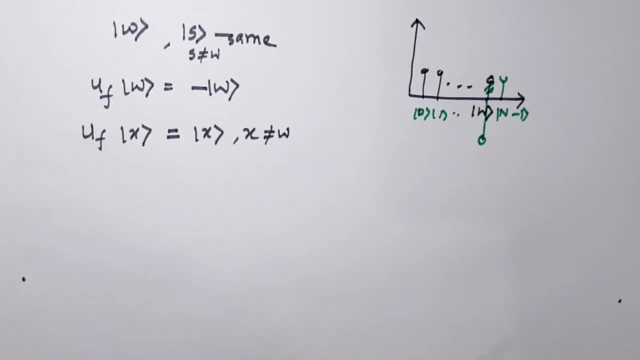 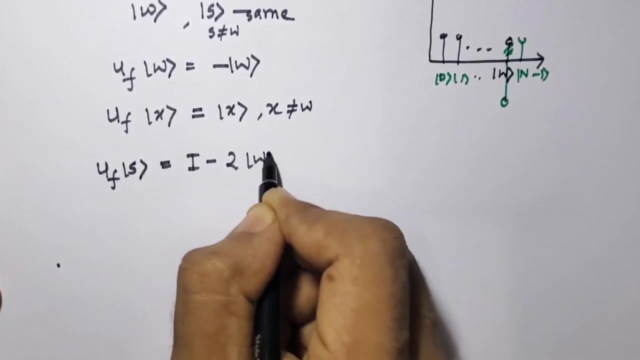 This change is done. This is my 0,, 1 or other states amplitude. This change is done after uf is applied onto this. Uf is defined mainly in this way: Uf of s is equals to i minus 2 times projection of w onto s. 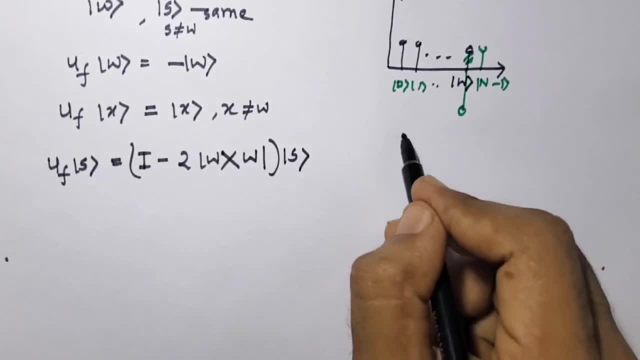 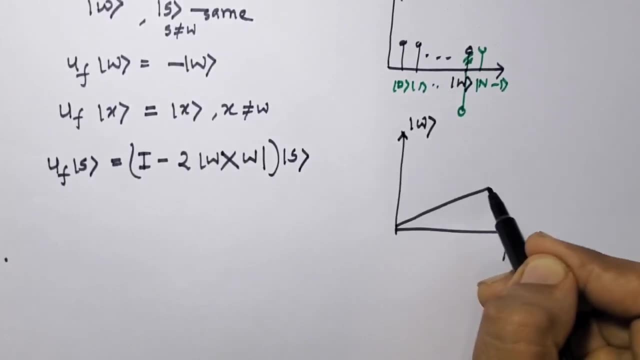 So let's see the phase diagram of it. In our phase diagram we had w in this side, w perpendicular in this and s in this. The angle was theta by 2.. So what happens? here? We see the projection of s onto w. 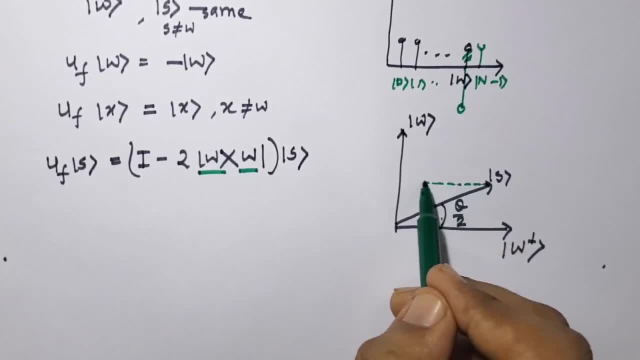 We take it twice, So the projection of s onto w is this, And this is the first one. If we subtract it again twice, it comes to this and this. So the new position is this: This is my s Uf acting on s. 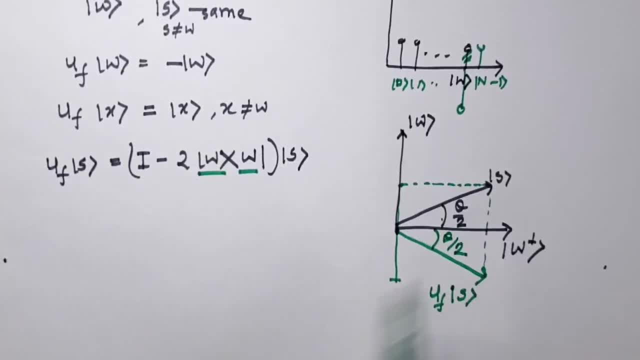 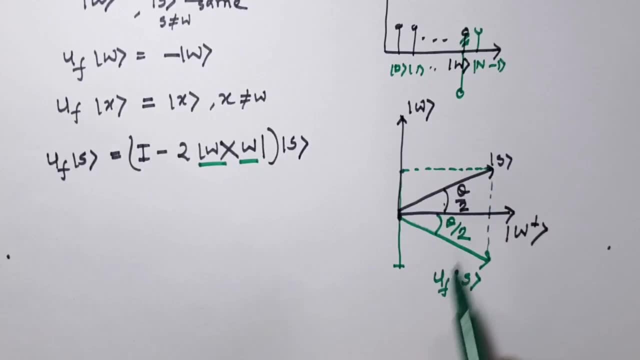 And this angle is similar to this one, theta by 2.. So you see the values of s, the projection of components of s along w perpendicular is not changed. They remain same. But the w states are now negative. They were like in this: 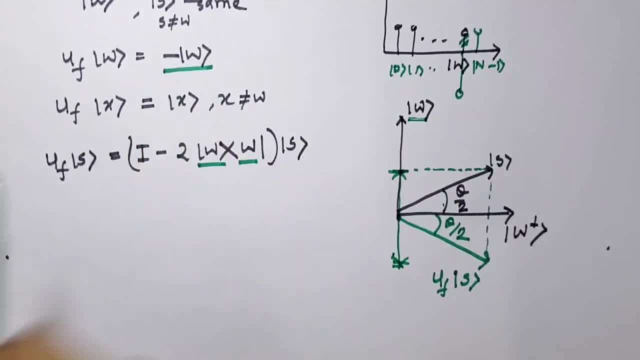 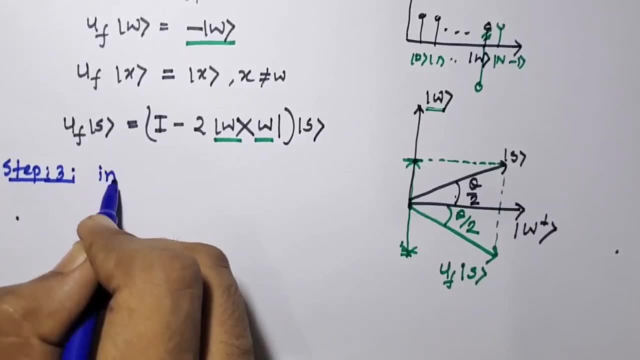 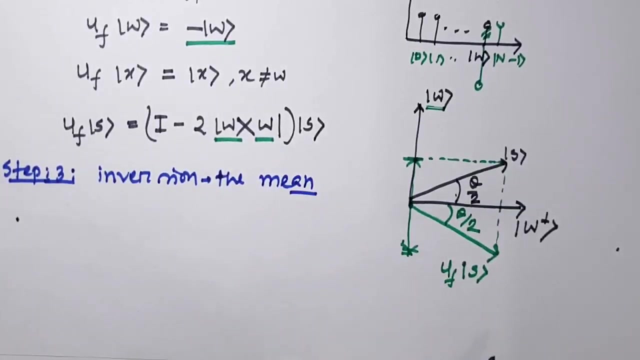 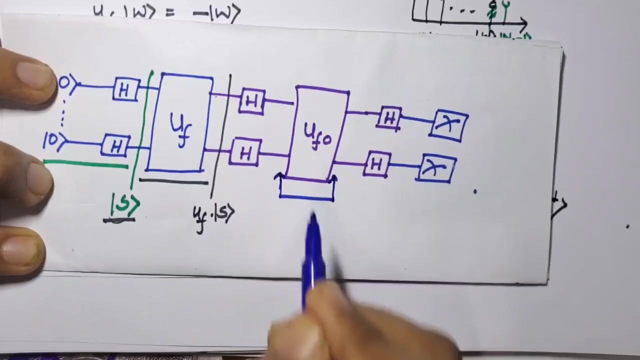 Now they are here. So phase change occurred only on w states. The next step is called step 3, which is inversion about the mean. So here we see the circuit. This is another oracle, And why and how these oracles work. 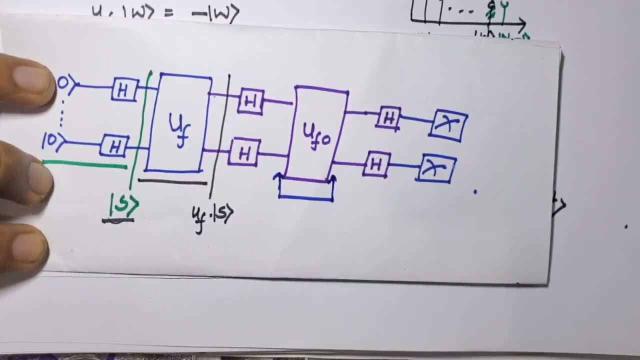 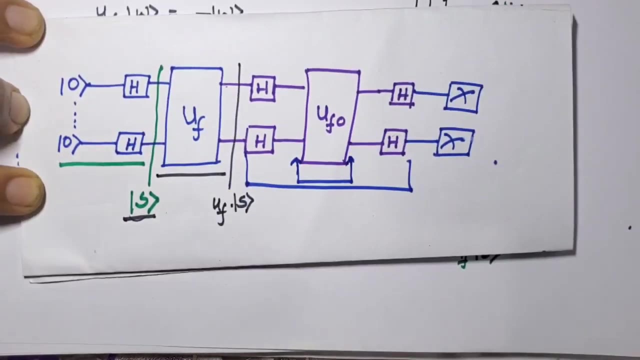 We have said earlier, these are mainly black box and physical devices. We insert queries and we get an output. The details we will discuss later, But now let's just concentrate on what are their functions. This oracle with these two hydromet gates performs an inversion operation. 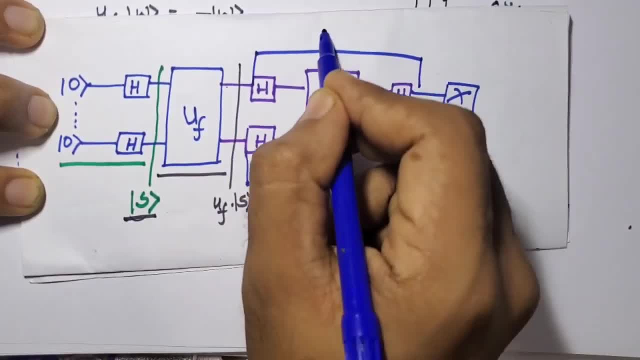 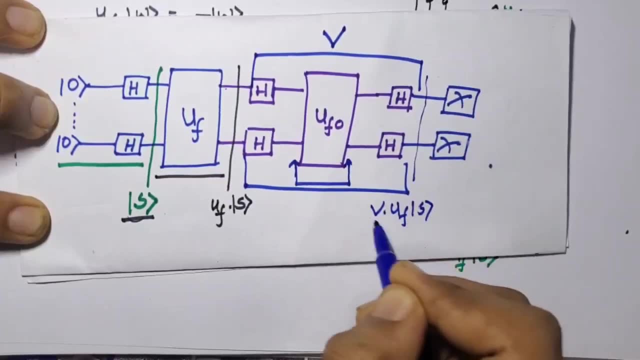 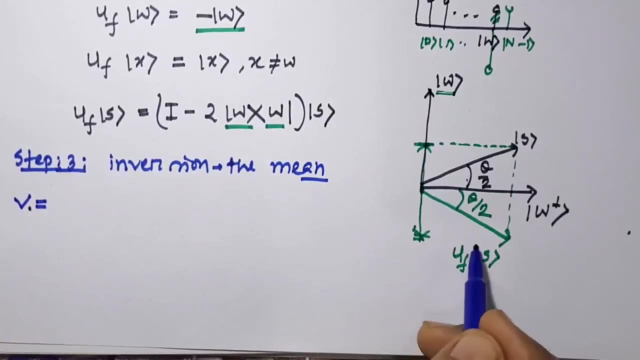 So it performs an inversion operation. This whole thing is we denote this as v and call the diffuser And after that we get the state vufs, v operator, your operator onto s. But the v is mainly projection of this one ufs onto s. 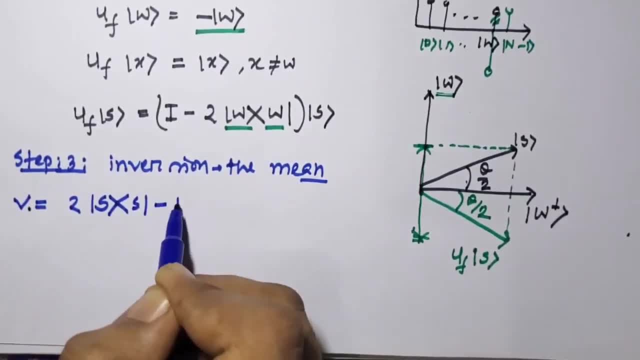 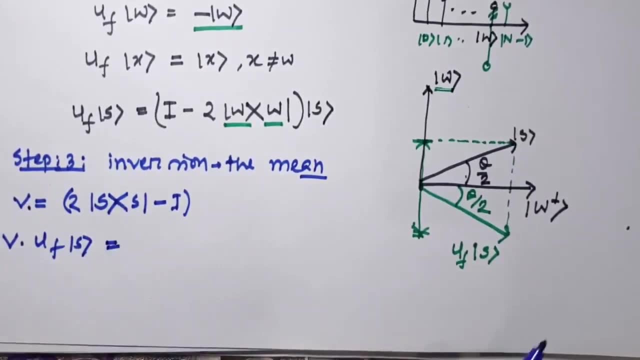 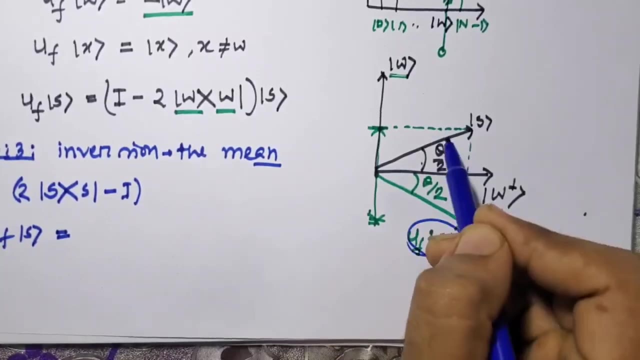 It is like this s minus identity matrix. So when we apply v on ufs, we get this. Let me show this in figure: We are taking the projection of this one onto s twice. So the first projection here, next again here. 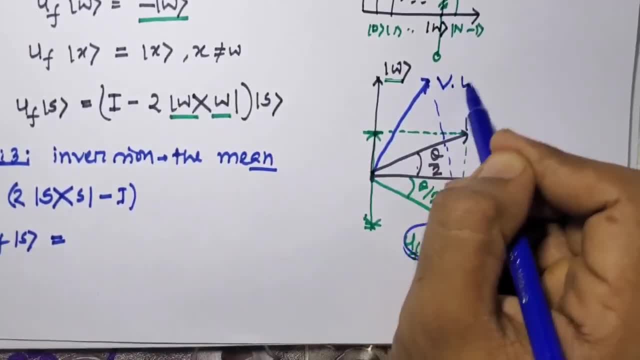 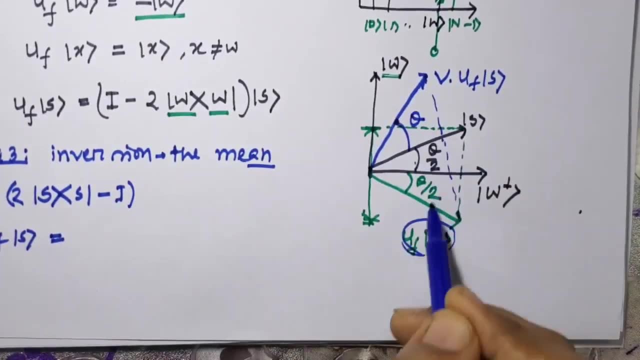 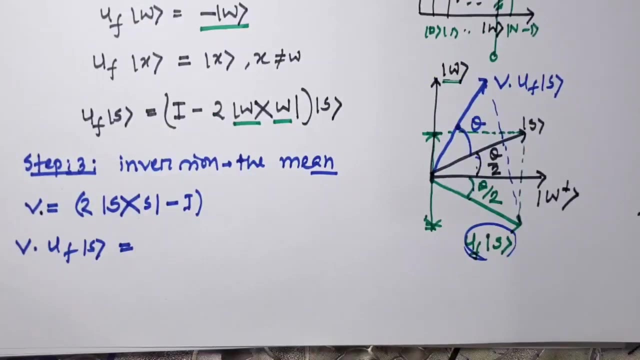 We get a new mistake here, which is vufs. So now, and this angle is theta, Because these two, the sum of these two, are theta, And the projection onto that side, this will also be theta. Now we see it was previously here- theta by 2 phase shifted. 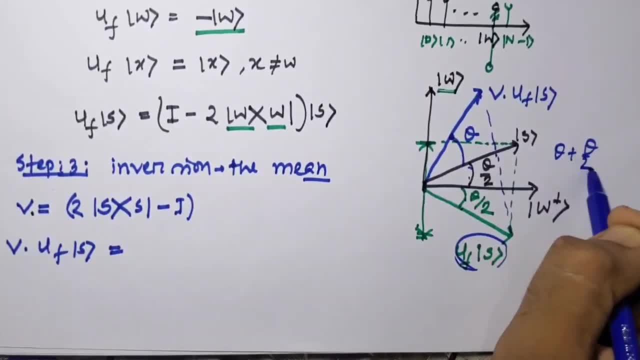 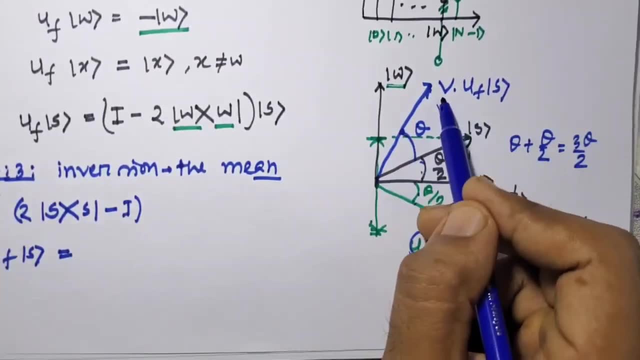 But now it's theta plus theta by 2, which means theta plus theta by 2, which is 3, theta by 2 shifted into that. So after one operation it is shifted. this What we do is in the Grover's algorithm. 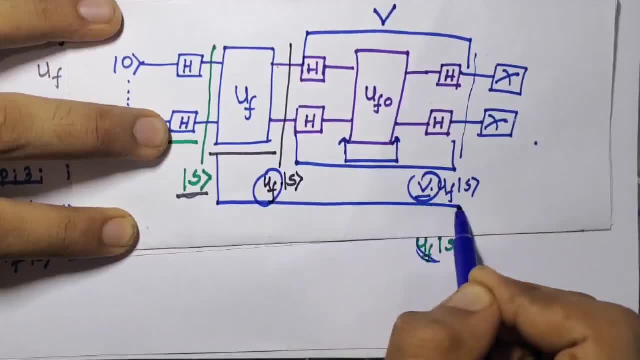 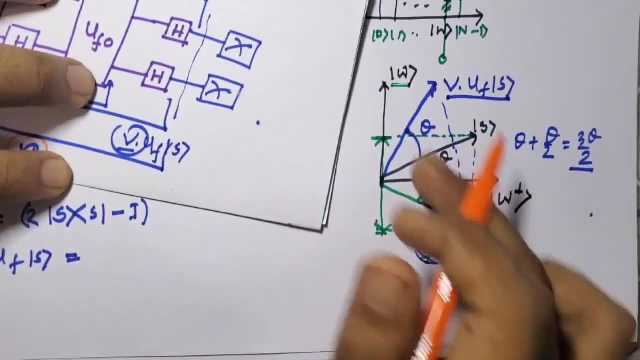 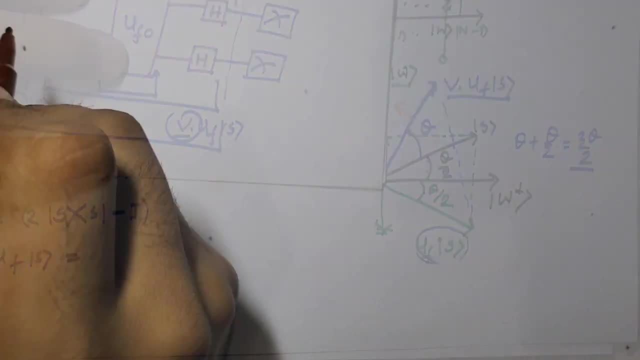 we run this uf and v this portion r times. We said it earlier, we run this r times. So every time this gets closed by theta into that side, It's shifted along w by theta every time. So we have decided that we will run this operation on s r times. 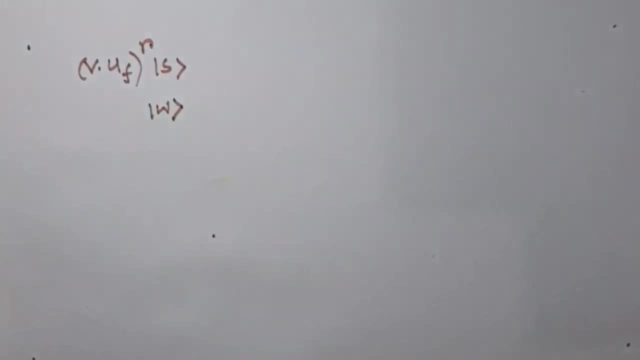 to get a high probability result of our expected w. So what is the value of r? let's say Here, if we draw the picture again w here, w perpendicular. here s was here And after two operations we got it here. 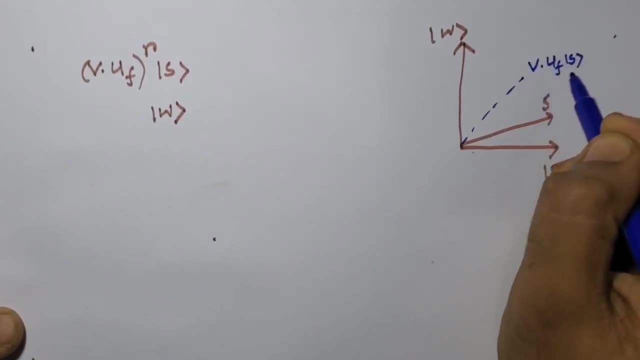 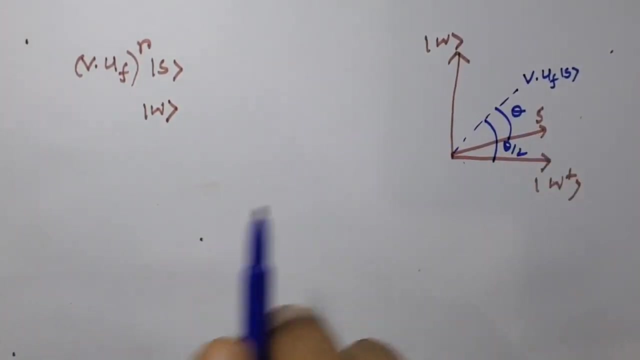 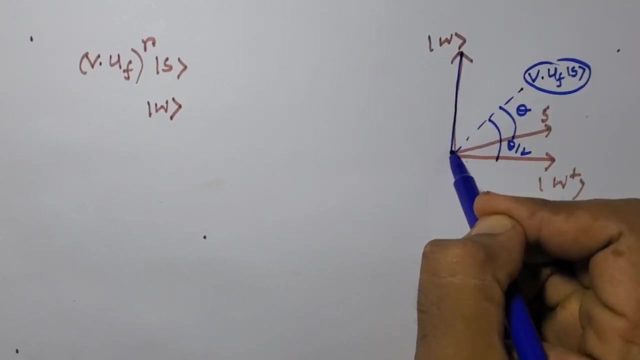 Let me write it blue v? uf on s After one one time operating v? uf. So the angle is now theta by 2 plus theta. What we want at the end, We want this to be aligned with this one in this side very close to w. 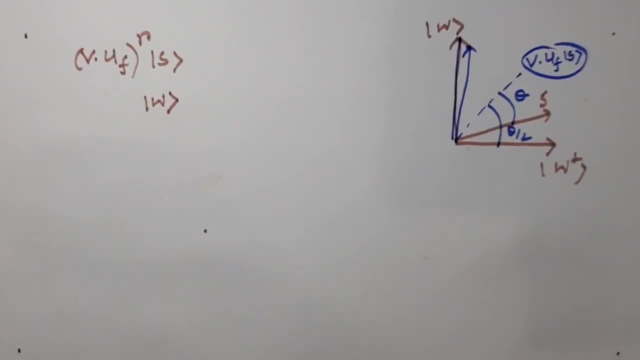 So we have the maximum probability of w. So when we will get that? We will get that when this angle is pi by 2.. Now it's 3 theta by 2. It will be pi by 2.. So and what? after every iteration, the angle increases by theta. 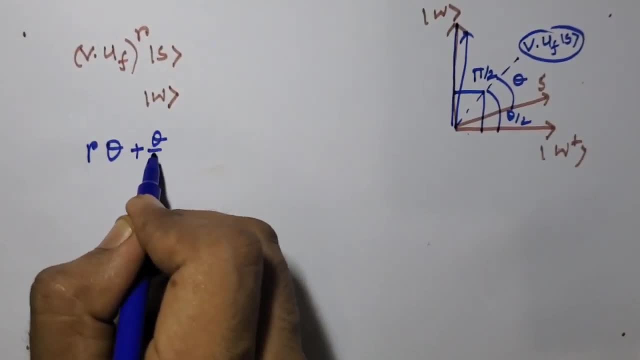 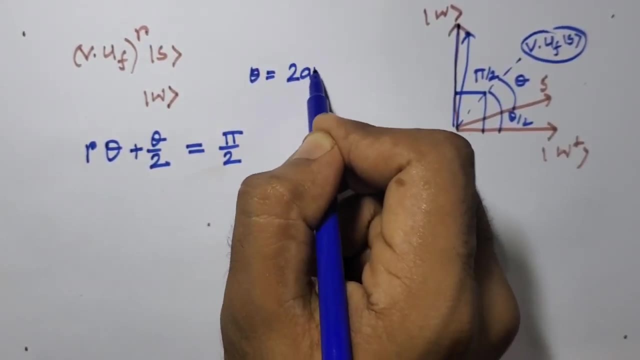 So after r iterations it will be r theta and the initial theta by 2.. We want this to be as close as possible to pi by 2.. Where We define earlier theta is 2r sine, 1 over root, 2 to the power, 2 to the power n.